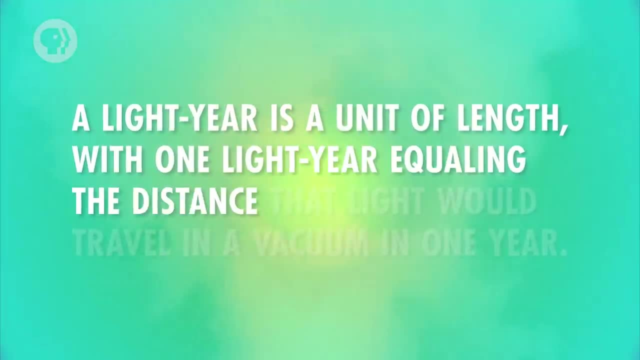 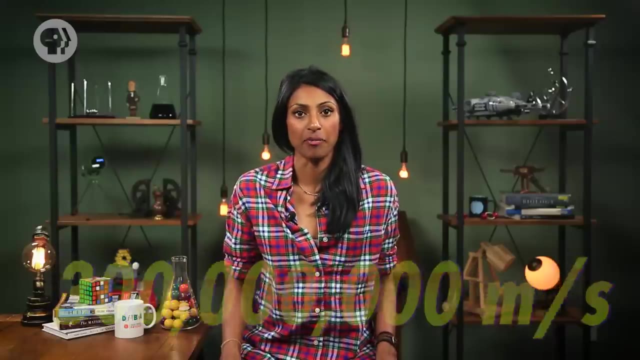 A light-year is a unit of length. with one light-year equaling the distance that light would travel in a vacuum in one year If you take the speed of light, about 300 million metres per second, and multiply it by how many seconds there are in a year. 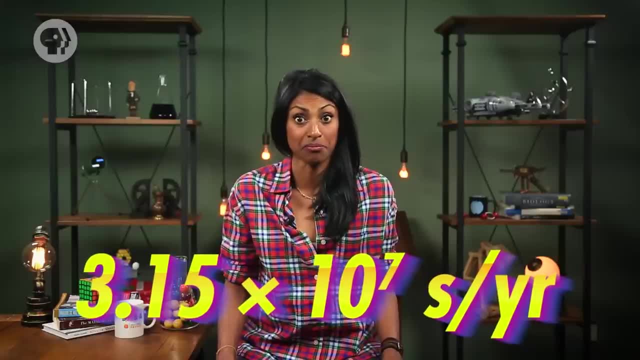 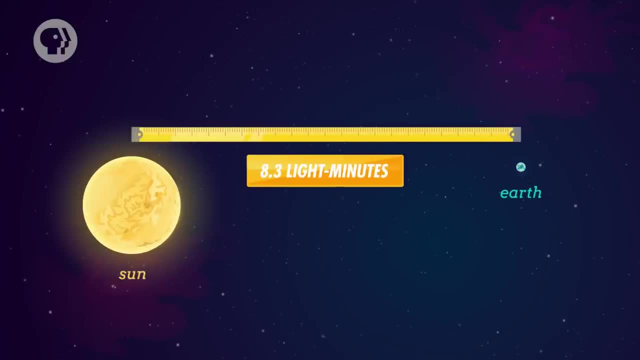 you find that one light-year is approximately 10 to the 16th metres, or 10 to the 16th metres, That's 10 million billion metres. To give you a sense of scale, it takes light just over 8 minutes to travel from the Sun to the Earth. 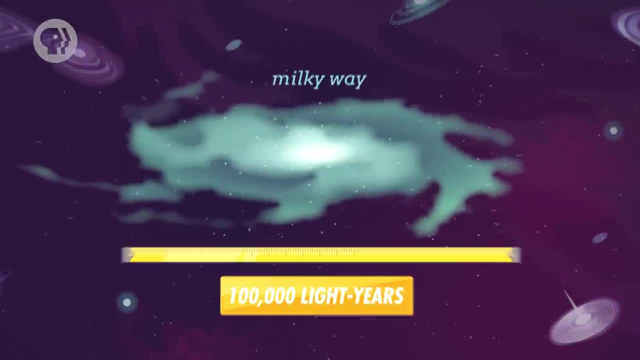 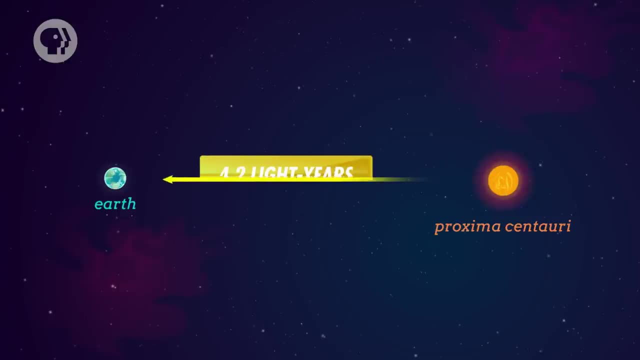 and the Milky Way is roughly 100,000 light-years in diameter. Sometimes we also use a unit called a parsec, which is equal to 3.26 light-years. Now, when we say that Proxima Centauri is 4.2 light-years away, 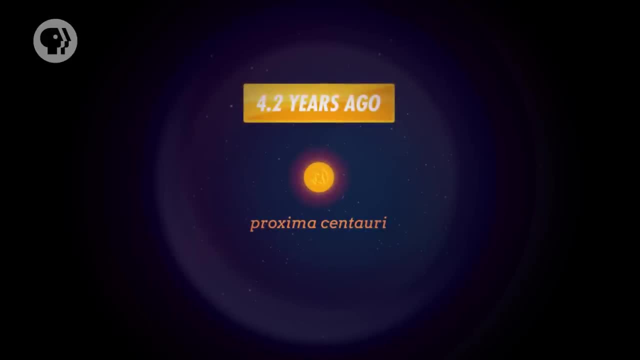 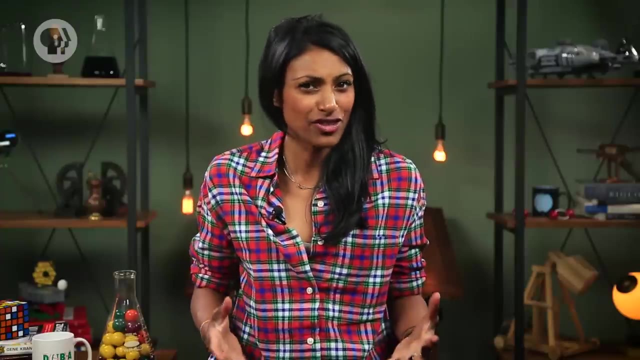 this also means that when we look at the star through a telescope, we're seeing what Proxima Centauri looked like 4.2 years ago. It takes light that long to get here from Proxima Centauri, so we'll never know what that star, or any star or other distant object- 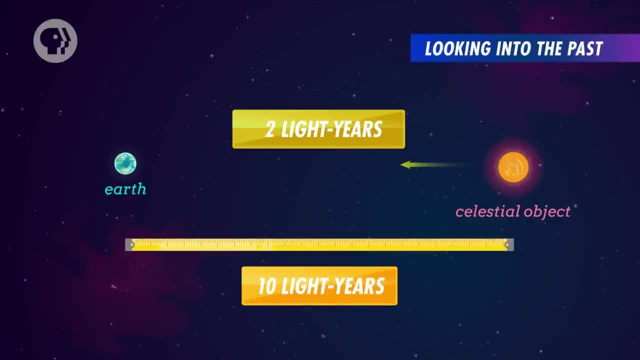 looks like at this exact moment. This means that, as we observe celestial objects far away, we're looking into the past, seeing what stars and galaxies looked like millions, if not billions, of years ago. While we're observing these stars, we can use a spectrometer. 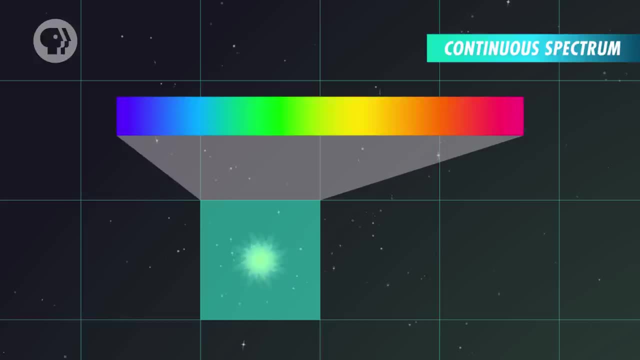 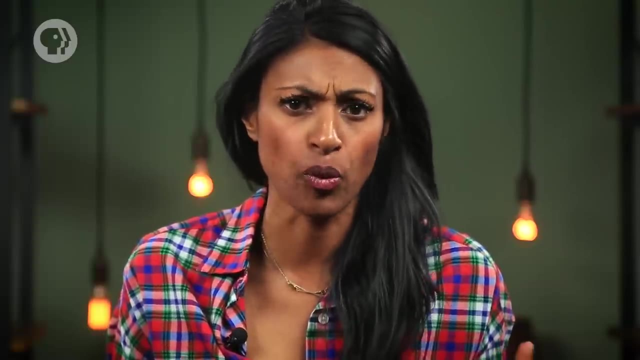 the device that separates wavelengths to reveal the star's absorption spectrum and its elemental composition. But when we study very distant bodies, we find that their absorption spectrum is slightly different from what we'd expect, given our knowledge of typology. We can also use a spectrometer to measure how much light is emitted by an object. 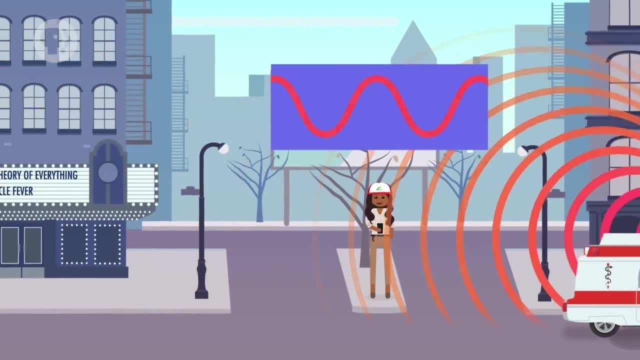 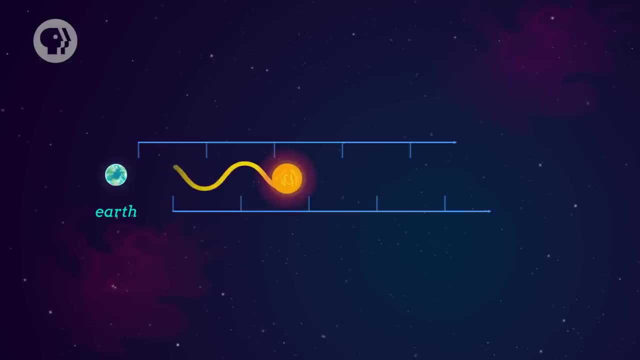 moving away from Earth and how much light is emitted by an object moving away from Earth. This is called the Doppler effect or the Doppler effect, which is a very typical star composition. Remember the Doppler effect: How the pitch of an ambulance siren becomes higher as it approaches you. 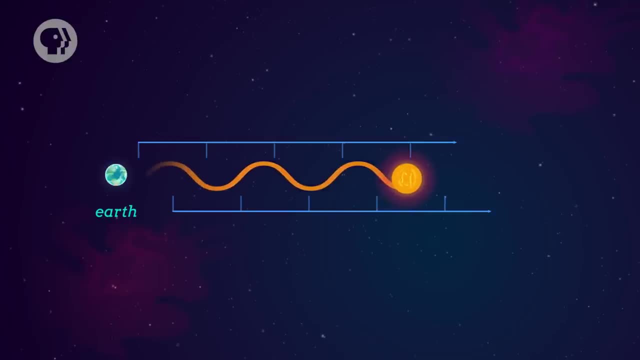 and lower as it moves away. The same effect happens with light. If an object is moving away from you, the speed of light doesn't change, but the peaks of the electromagnetic wave that it emits move further apart. This effect, which occurs with light emitted by an object moving away from Earth, 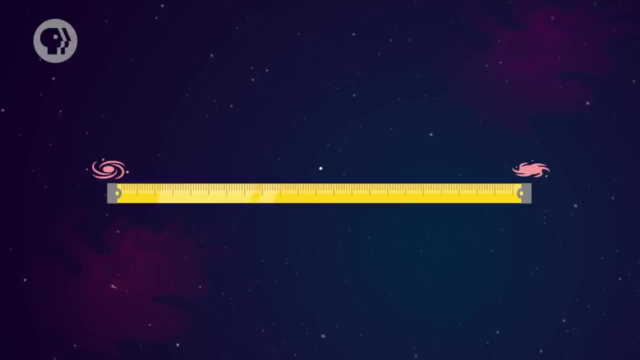 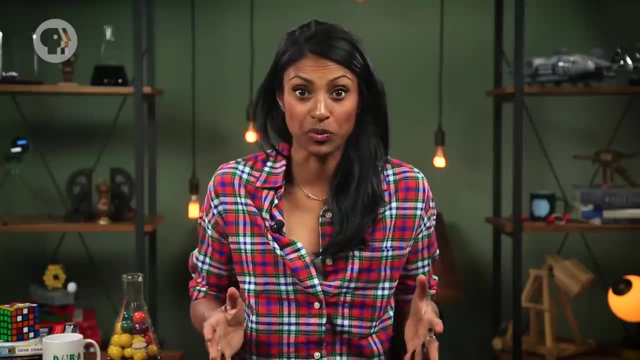 is called the Doppler effect or the Doppler effect. The Doppler effect, which occurs with light emitted by an object moving away from Earth, is called the Doppler effect. And if that wasn't strange enough, astronomers such as Edwin Hubble. 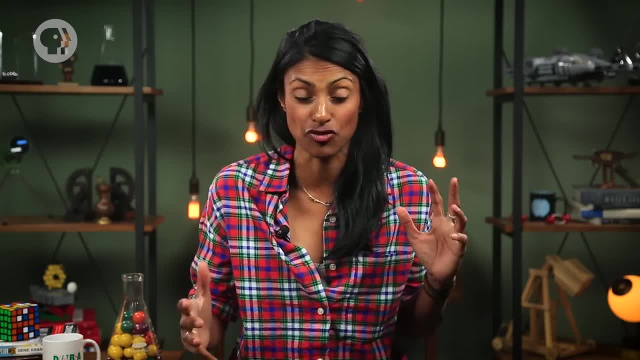 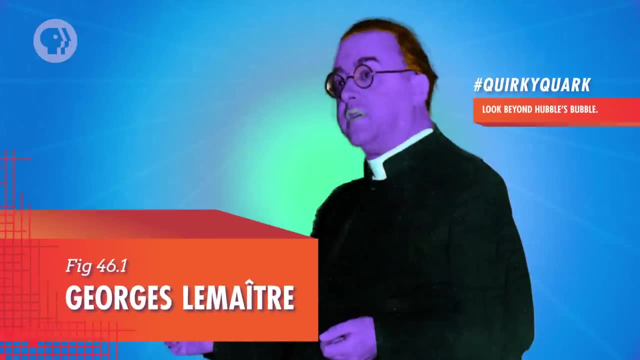 noted that the amount of redshift is proportional to the distance from Earth, So the farthest galaxies are moving away even faster than the close ones. Georges Lemaitre, a Belgian physicist, proposed this relationship as Hubble's law. It expresses the velocity at which a galaxy is speeding away from Earth. 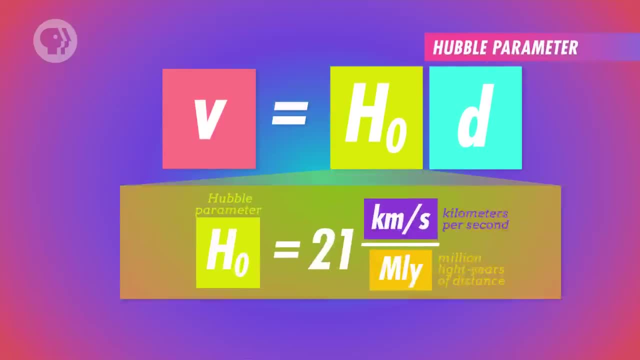 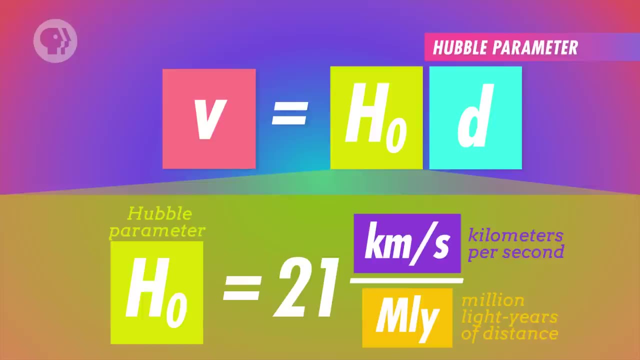 in terms of its distance from us. The equation uses a proportionality constant called the Hubble parameter, which says that for every million light-years of distance from us, a galaxy is moving away at an additional 21 kilometers per second. Now, the fact is that nearby galaxies might be going away from us or towards us. 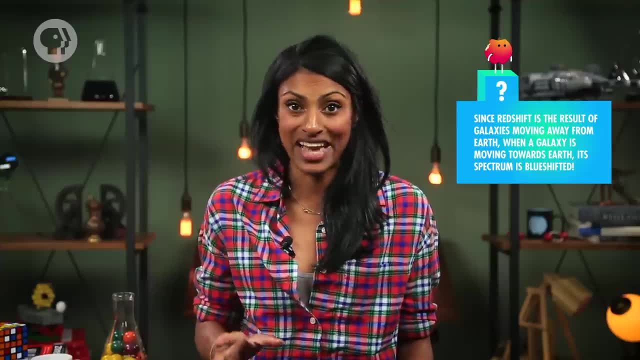 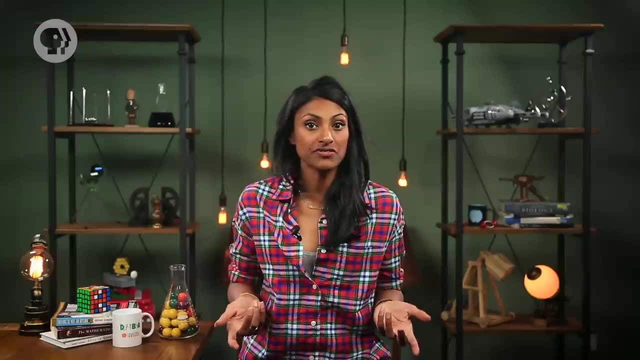 based on how they're moving within their local cluster, But the overall tendency for distant galaxies to recede from us is much more common. so Hubble's law holds true in most cases And this trend of distant galaxies moving away from us and from one another. 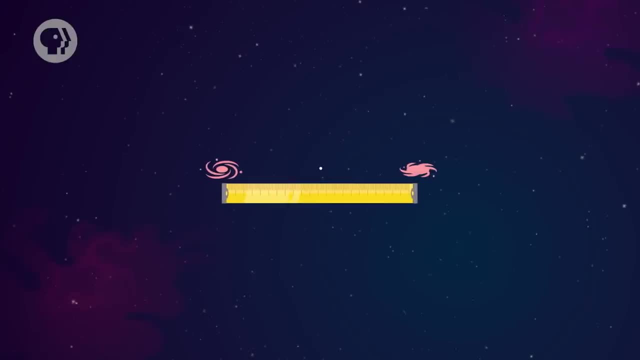 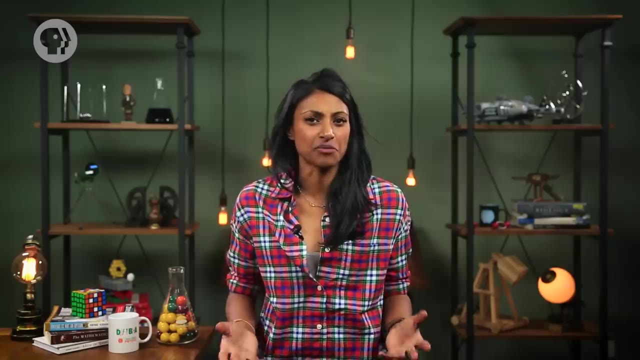 is called cosmological redshift. By the way, this expansion looks the same whether you're on Earth or not. No matter where you are, all distant galaxies appear to be moving away from you, So this leads physicists to believe that at some point in time, 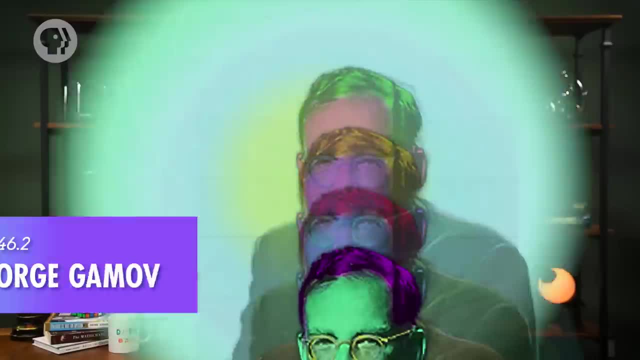 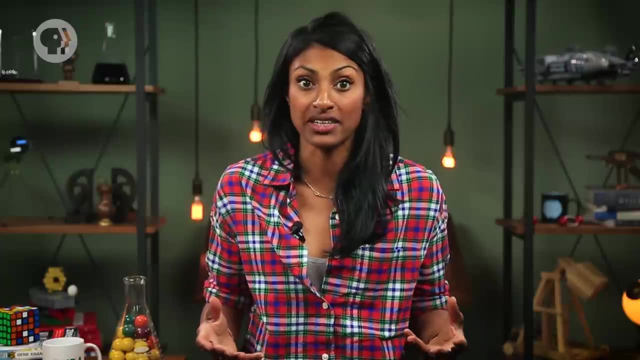 all the stars and galaxies were closer to one another- A lot closer. In the 1940s and 50s, Russian-American physicist George Gamow developed a theory of the early universe that explained, among other things, why so many light elements like hydrogen and helium. 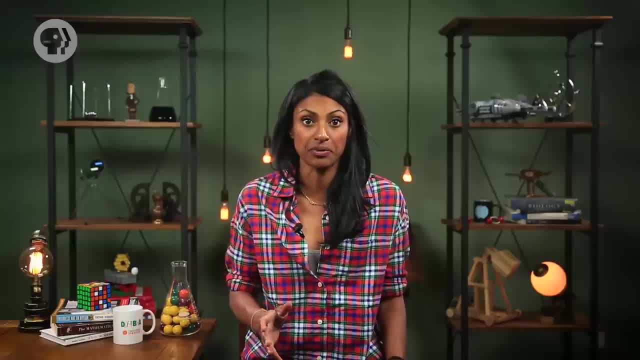 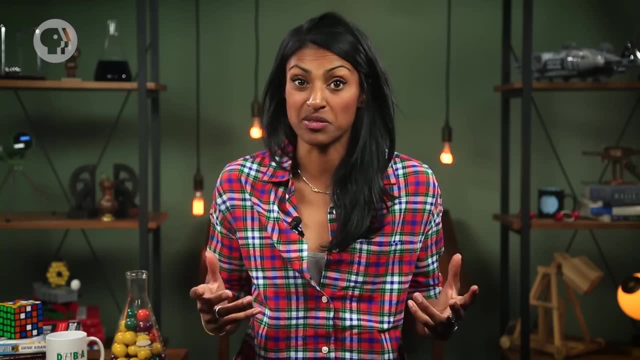 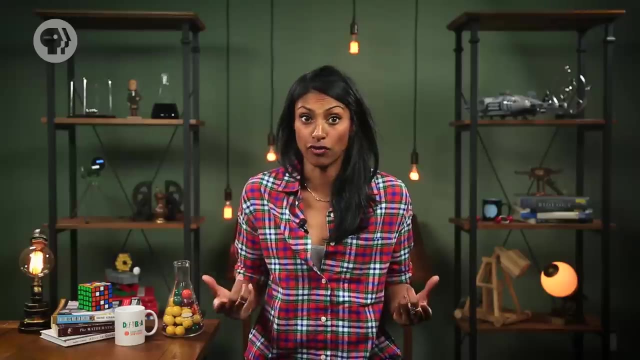 were observed throughout the cosmos. This theory suggested that the universe began in a state of highly compressed hot plasma, a sort of hot soup of elementary particles. His theory became known, somewhat dismissively, by his colleagues, as the Big Bang theory, And this same theory ultimately predicted that there should be radiation left over from 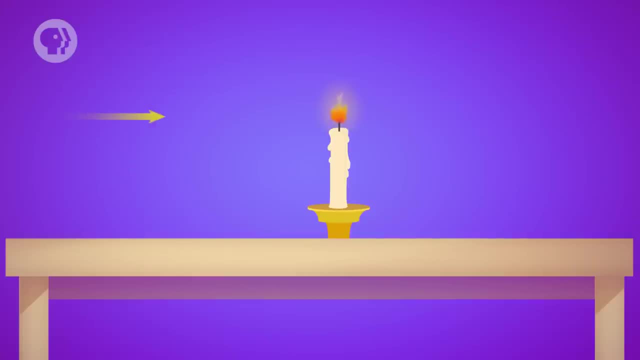 the initial rapid expansion of that compressed plasma. This is because hot plasma, like the plasma in the flame of a candle, is not transparent, But ordinary gas, like the air around a candle's flame, is transparent and it lets light travel freely through it. 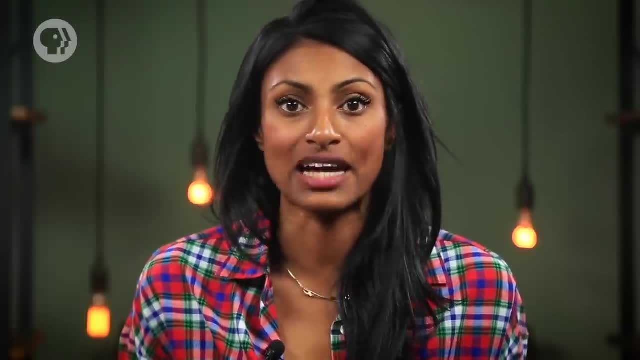 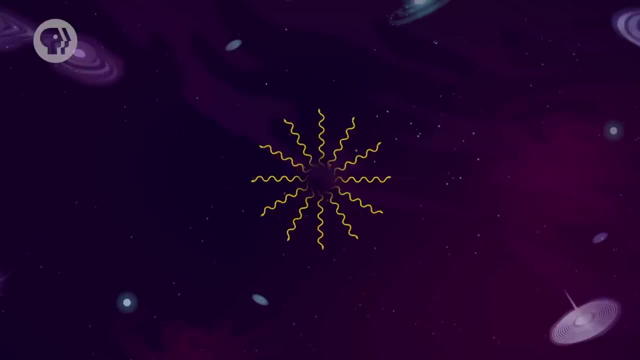 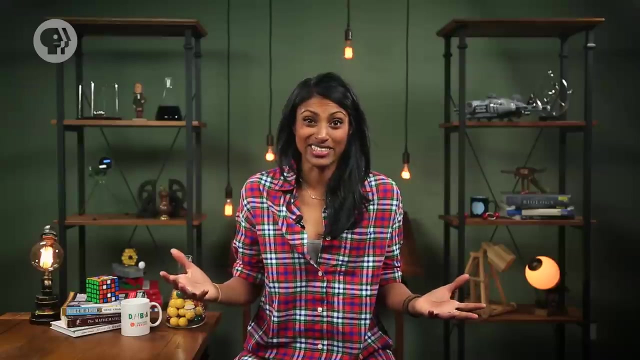 Gamow realized that the early hot universe was originally opaque until it cooled down to the point where it became transparent. Once that happened, the thinking goes light from. the Big Bang was able to travel freely, but its wavelength kept stretching out, redshifting until it could only be detected as microwave radiation. 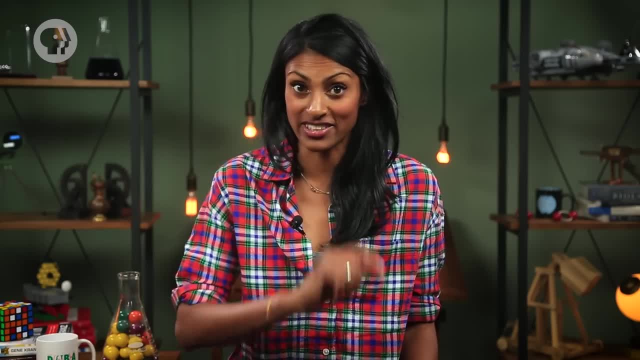 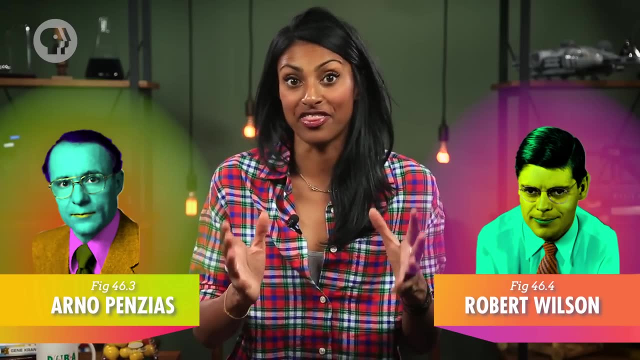 Gamow's theory didn't gain much acceptance and it was largely forgotten Until in 1964, American astronomers Arno Penzias and Robert Wilson pointed a radio antenna into space and discovered cosmic microwave background radiation. They basically discovered the radiation from the Big Bang by accident. 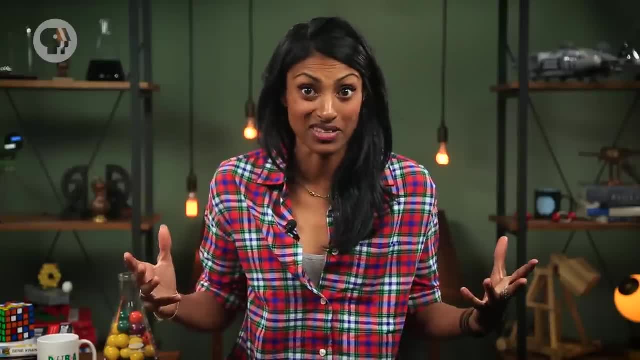 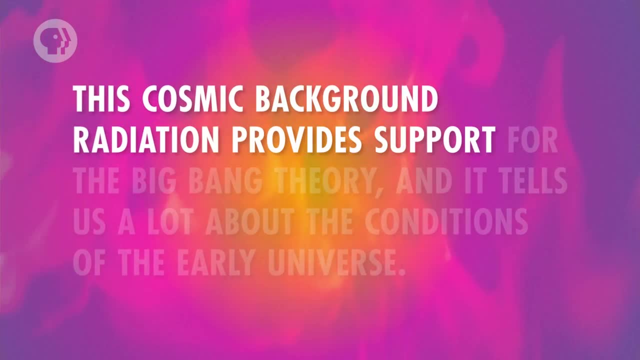 They found that low-energy microwave radiation persisted at all times, day and night, and they concluded that the source of the radiation was the universe itself. This cosmic background radiation provides support for the Big Bang theory and it tells us a lot about the conditions of the early universe. 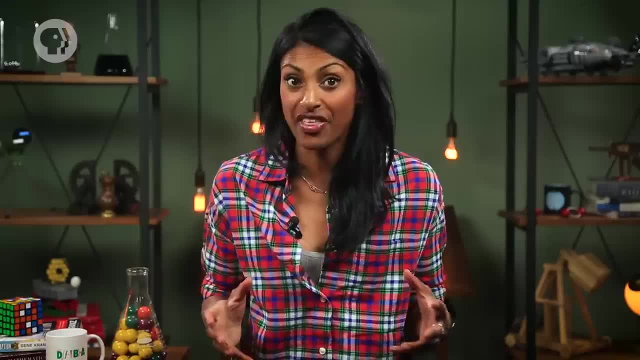 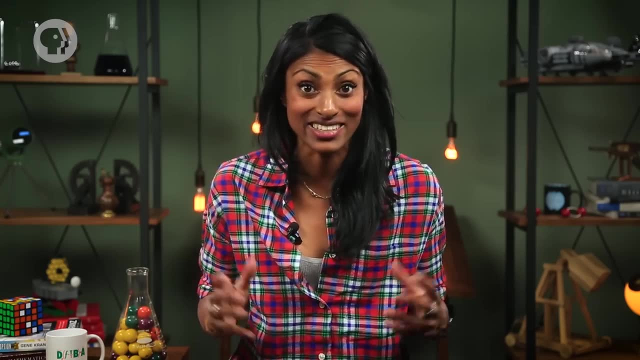 Thanks to these insights, along with the observed expansion of the universe and other evidence, we've learned that the universe began in a hot, dense state, then cooled and produced galaxies and clusters that we see today. However, many mysteries remain, For instance, if the universe started with such high density and temperature. 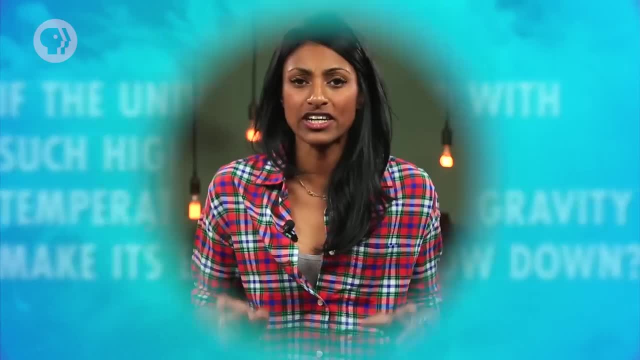 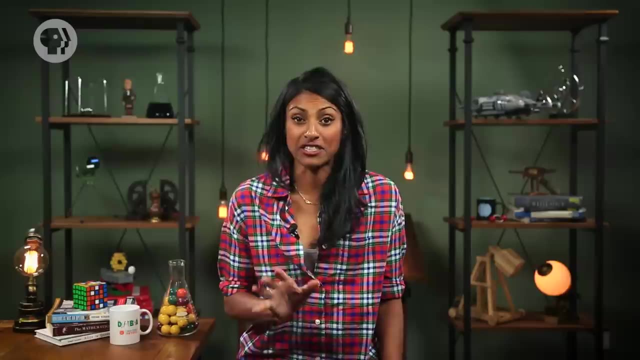 wouldn't gravity make its expansion slow down? The fact is, the rate of expansion would slow down only if the universe was filled with nothing but matter and radiation, But that's not the case. Space is filled with a constant, or at least slowly varying form of energy known as dark energy. 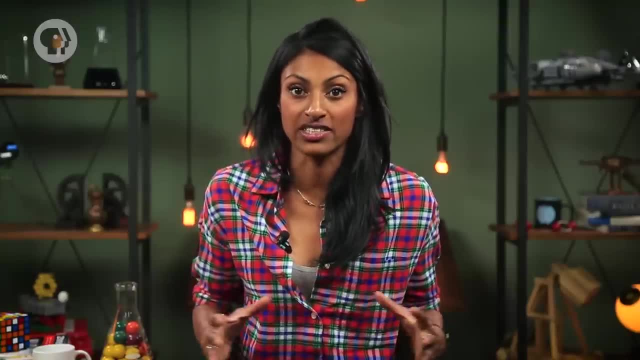 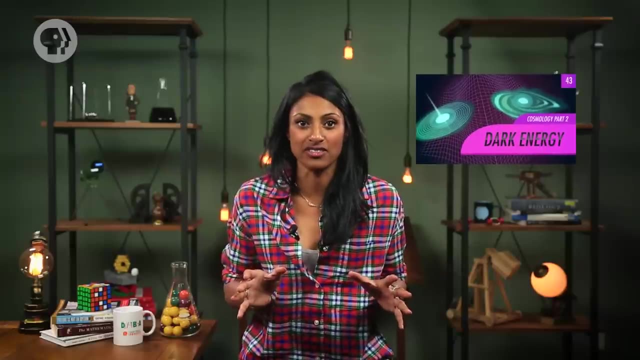 And because of the pervasive presence of this energy, according to General Relativity, gravity is actually causing it. It's actually causing space to expand and accelerate. This isn't just theoretical: Recent evidence suggests that the universe actually is accelerating in its expansion. 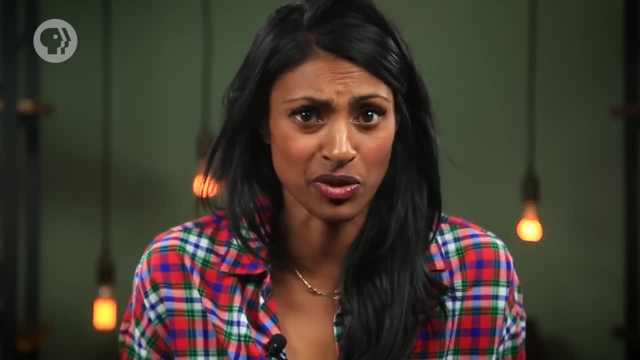 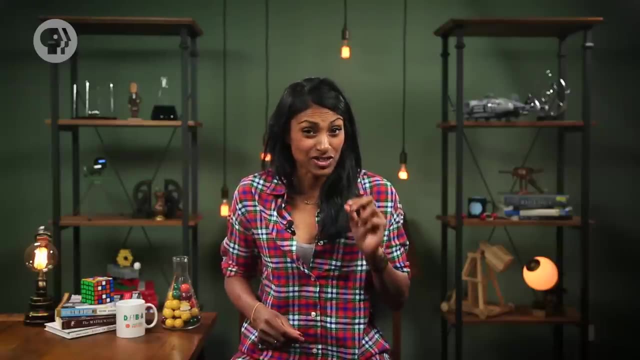 showing no signs of slowing down. But beyond the fact that it exists, there's not much that we know about dark energy. Another one of the universe's great mysteries is the existence of mass that we can't see, But we know that it too exists. 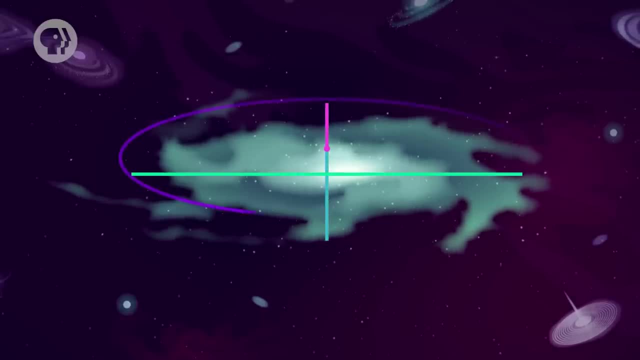 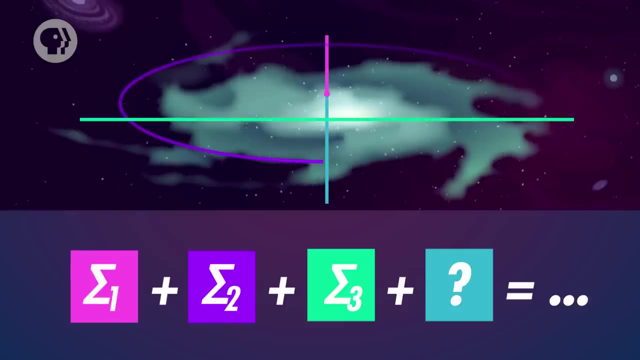 When we study a galaxy's rotation, we can estimate how much mass is in it by measuring its radius and rotational velocity. But when we actually calculate that mass, the result is far greater than what's observable as stars and gas. The conclusion is that there's an immense amount of mass in the universe known as dark matter. 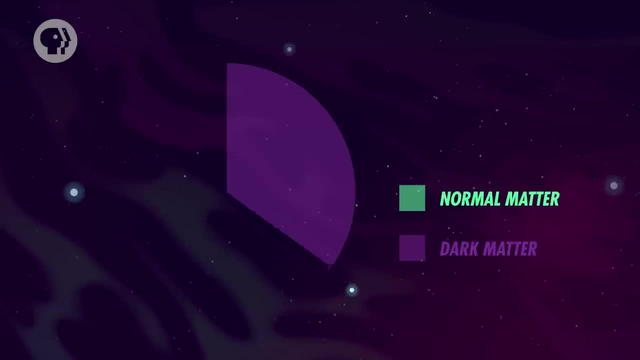 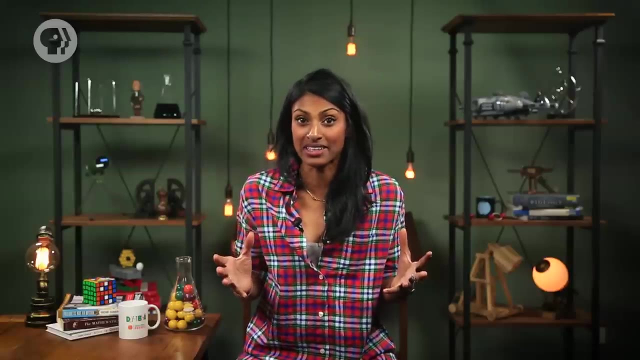 which doesn't reflect or emit any light. By current estimates, dark matter makes up almost 85% of all the matter in the universe. This means that all visible matter, including stars and planets, make up just a small percentage of all energy in the universe.